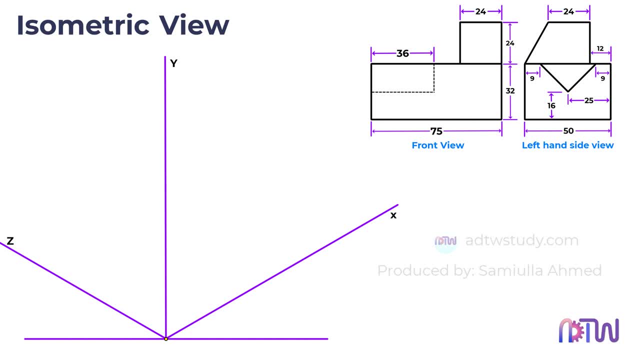 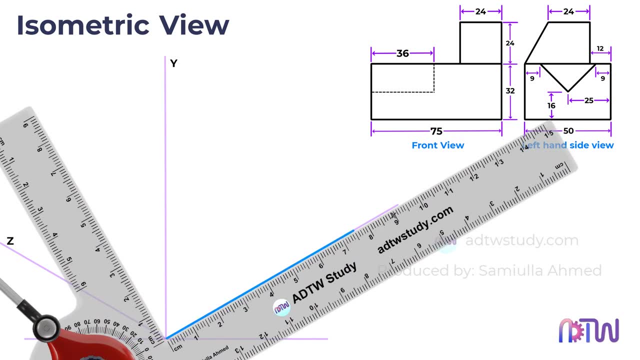 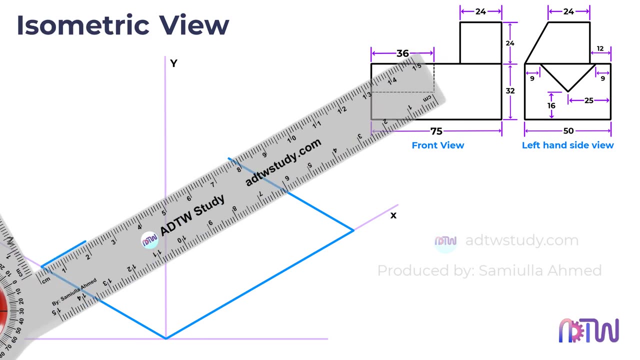 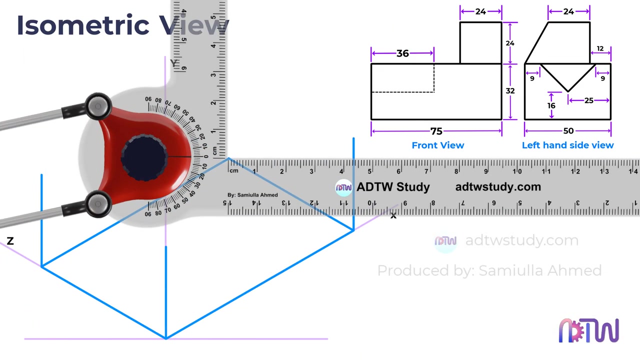 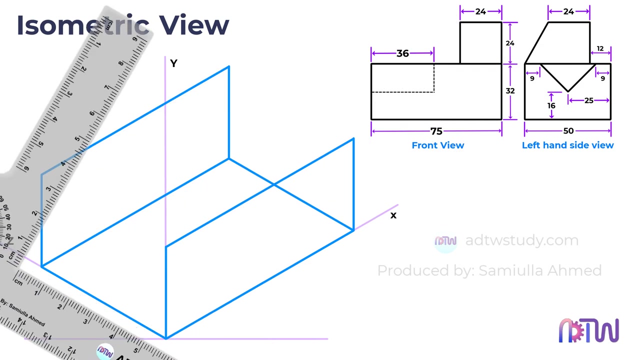 to create the outline for the base of the given object. To proceed, use a drafter and create the base outline, as demonstrated Now. let's focus on the top view of the object. Let's focus on the side view of the object, where we notice a distinctive V-shaped groove. 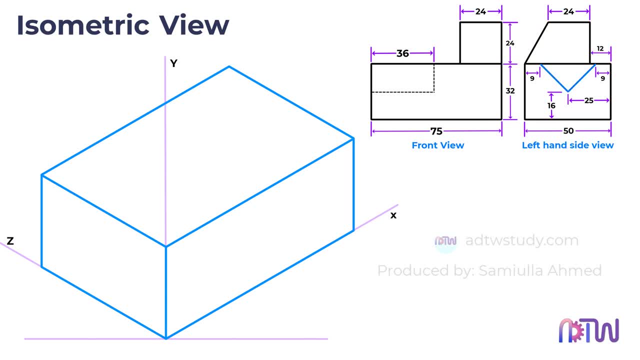 extending 36 millimeters along its length. To replicate this V-shaped groove, we will begin by dividing the side length into two equal parts, since the groove aligns perfectly with the middle of the side view. After this division, mark two points at a distance of. 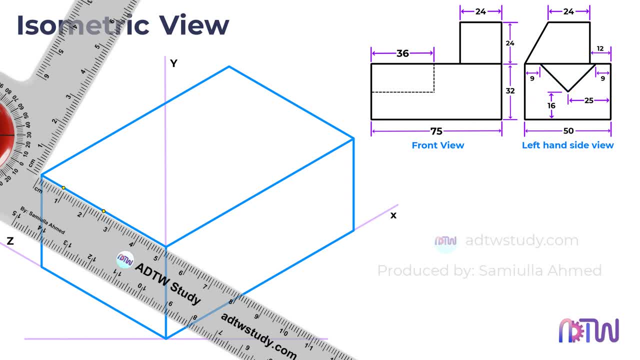 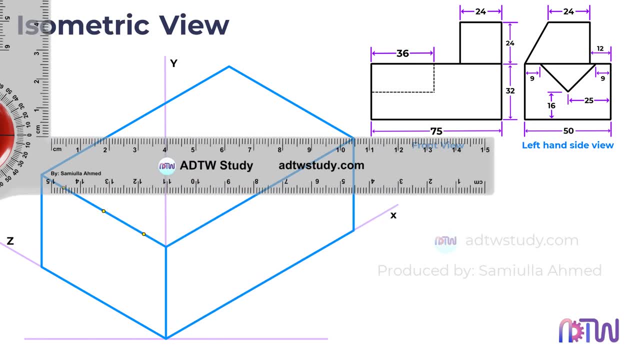 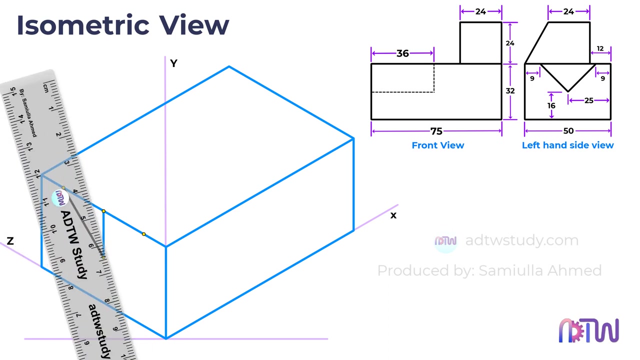 9 millimeters from the corners on each side. Now let's draw a vertical line. We will first make a vertical line that spans 16 millimeters downward from the center point you established earlier. The end point of this line will serve as the third point To complete the construction. connect these three identified points. 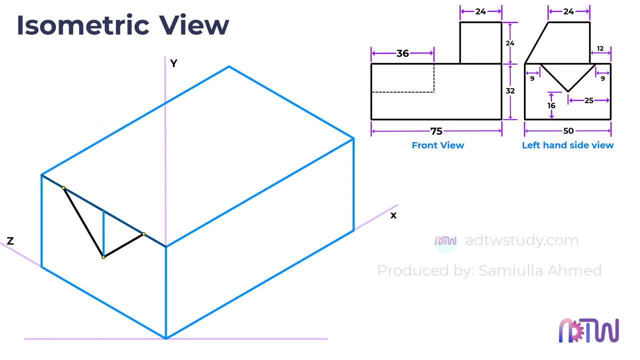 This will effectively recreate the V-shaped groove within the side view. Following this, your next step involves extending this groove by 36 millimeters along the length. To achieve this, draw lines that are 36 mm in length, parallel to the X-axis, from each of these three corner points. 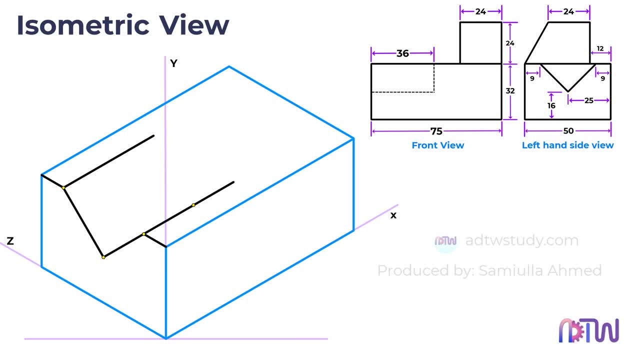 Finally join the endpoints of these extended lines to seamlessly finalize the detailed groove. And there you have it: the base of the given orthographic views is now complete. The next step involves completing the top portion of the object, Observing the dimensions. the bottom of this top section features a length of 24 mm and a width of 38 mm. 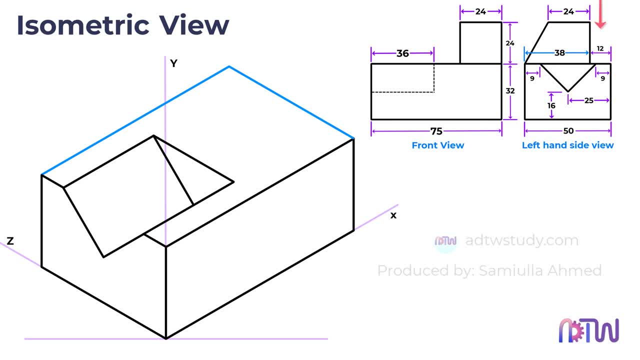 You can deduce this by subtracting 12 mm from the total width of 50 mm, which accounts for the overall object width. Now, shifting out of the top portion of the object, you can see that the top portion of the object is now complete.